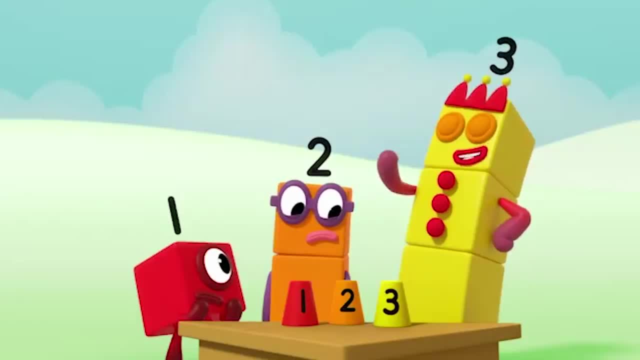 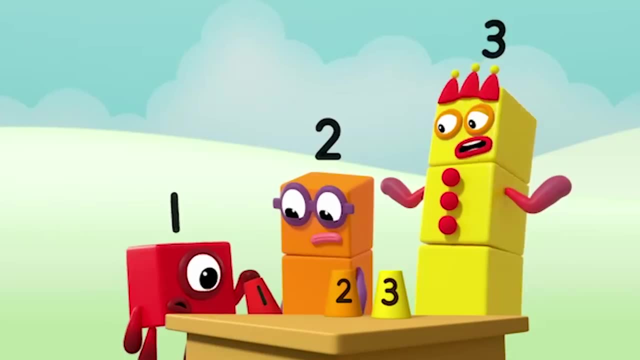 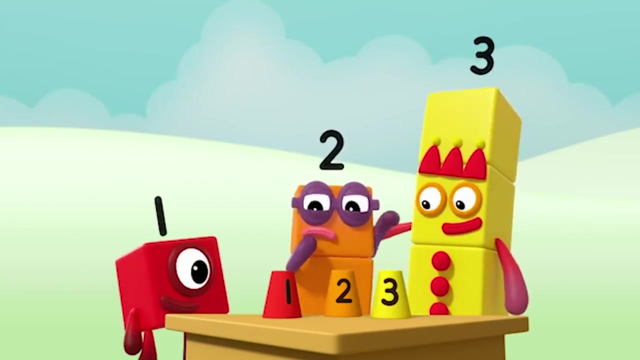 One: You're the first number, so you can have first guess This. one, The first cup. Oh, Bad luck. one, Two: You're the second number, so you get second go. Oh, This, No, That. 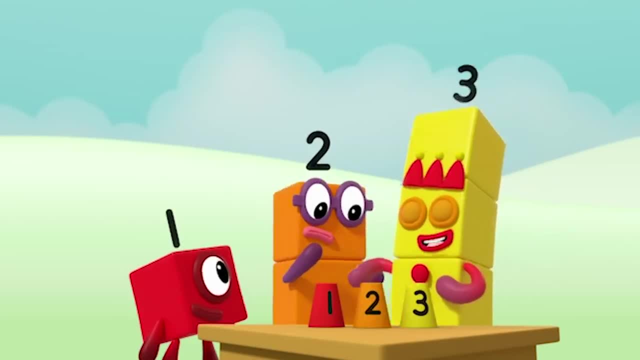 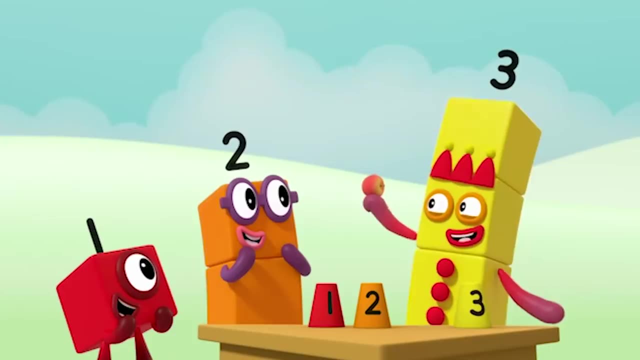 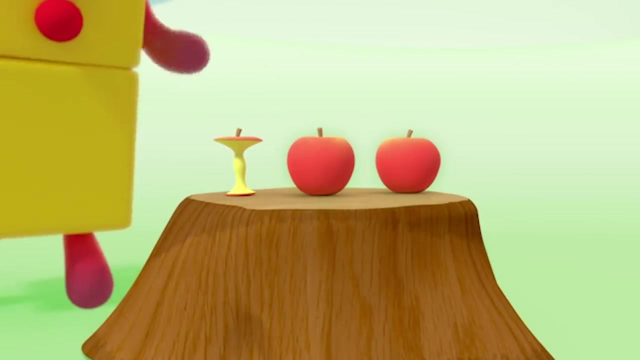 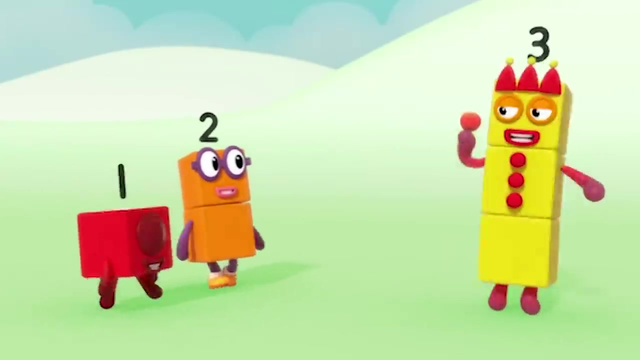 Oh, Oh, My turn. Three is the third number. Add one, two, three, Third time, lucky, Yay, Well done. One apple gone, Two apples left, Let's play again. Let's play apple on top, Oh. 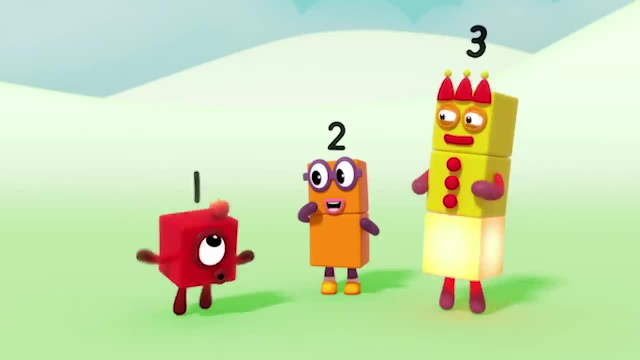 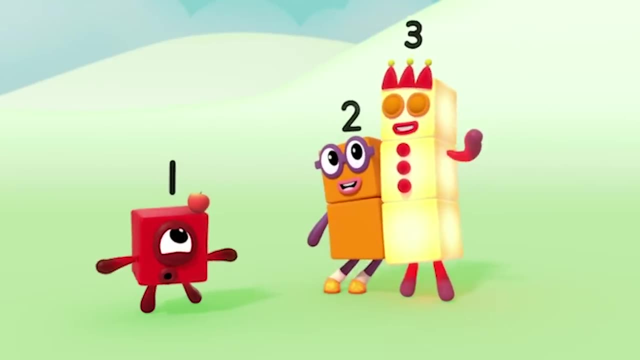 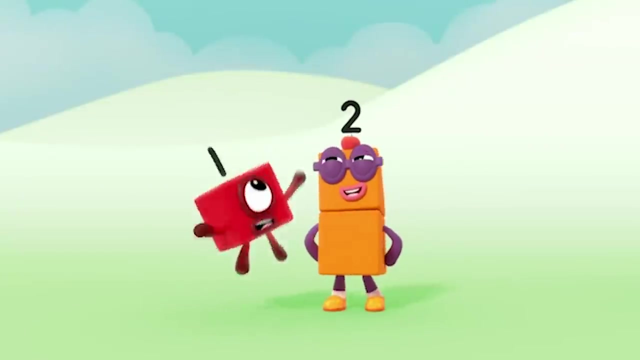 Three simple rules: Apple on top. Don't let it drop. Now try and swap. Hey, I can't reach. I'm smaller than you. I'm the smallest number, Then I'm bound to win. I'm bigger than you. 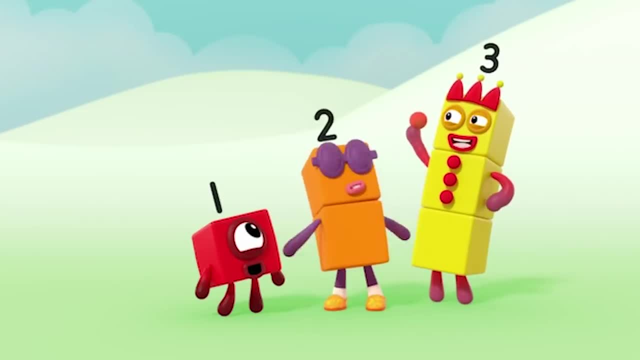 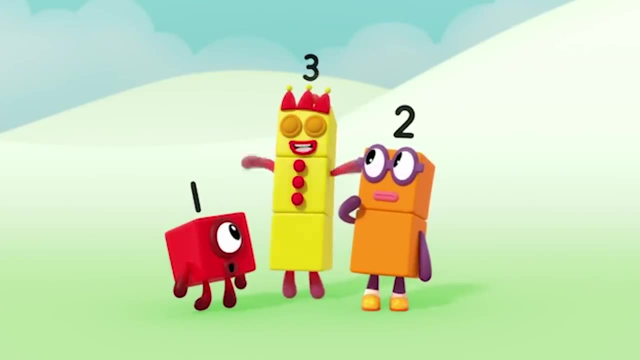 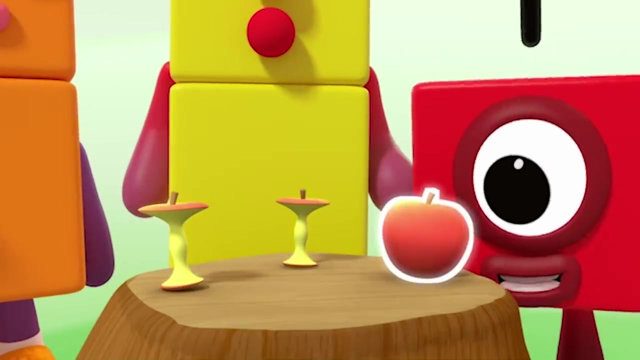 Oops, Silly me. I'm bigger than one, but smaller than three. I'm bigger than both of you, I'm the biggest. So I guess I win again. One, two, three, Two apples gone, One apple left, Surprise. 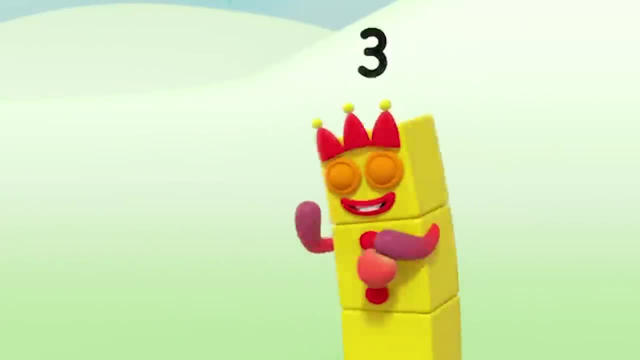 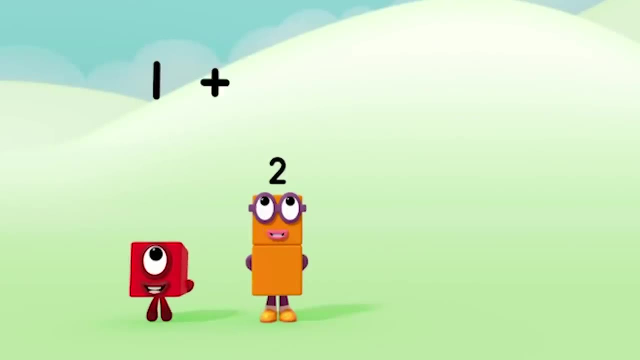 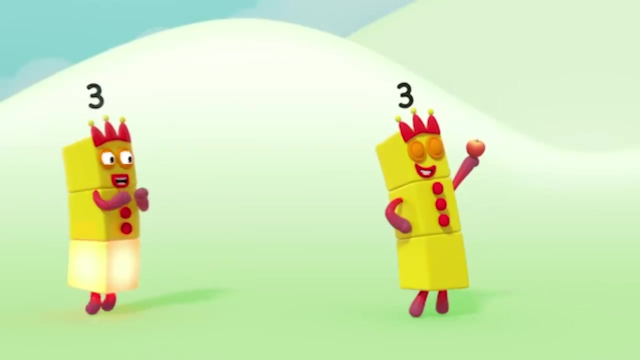 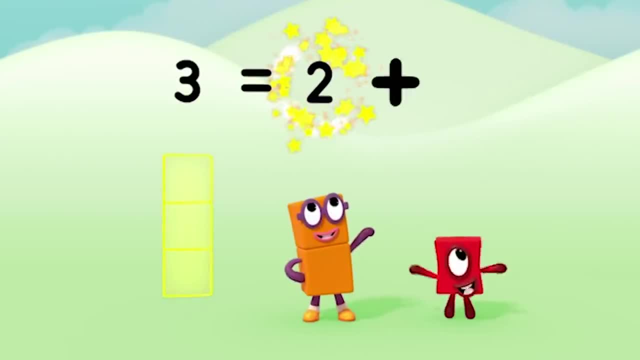 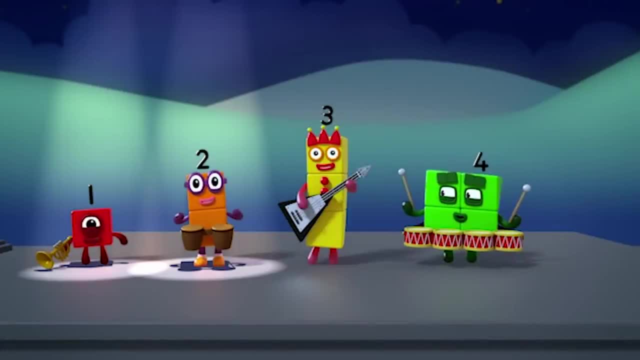 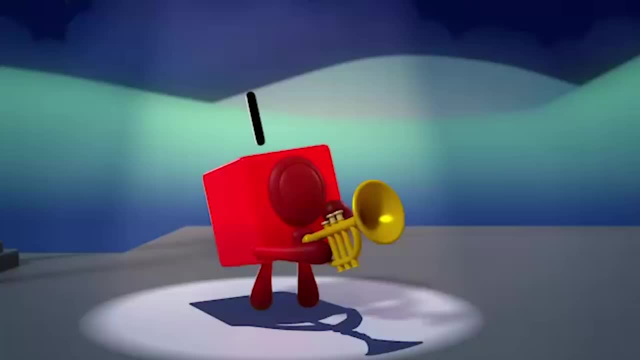 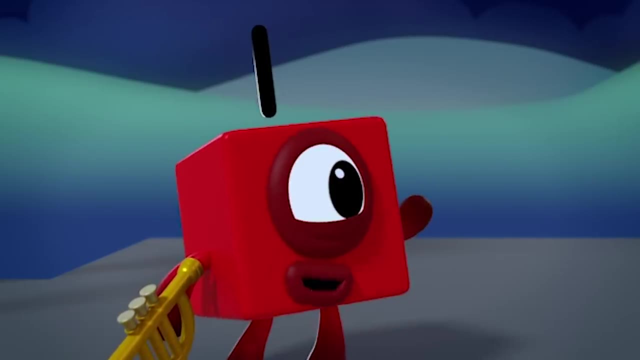 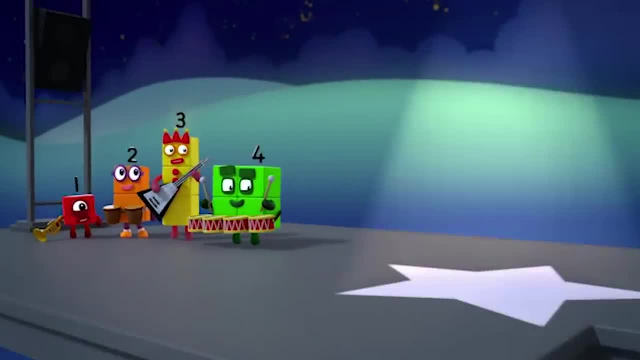 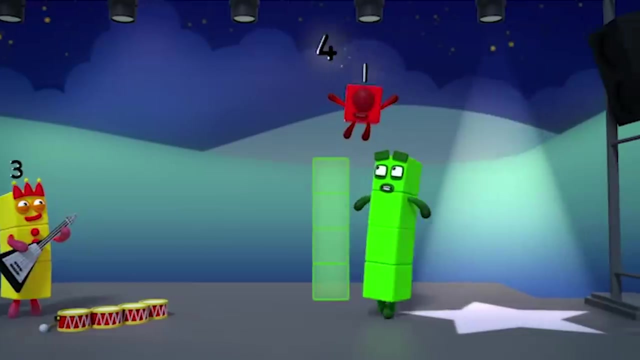 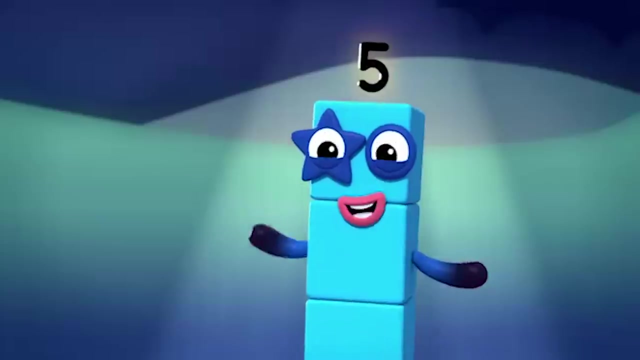 Make a wish. Oh, it's star-shaped. Who's it for Me? Well, I'm the biggest, I'll go first. Or Plus one equals five, I am five, I feel so alive. One, two, three, four, five. 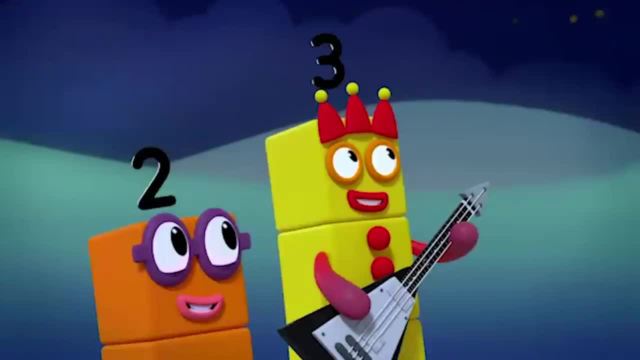 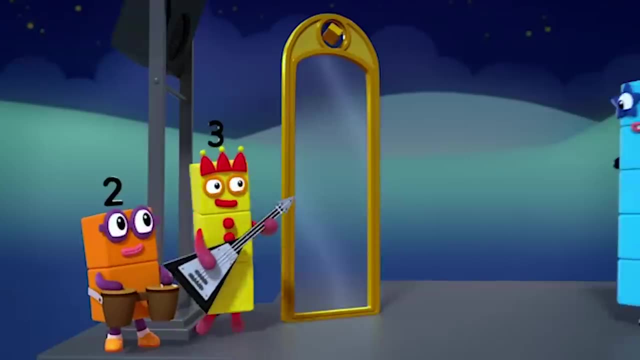 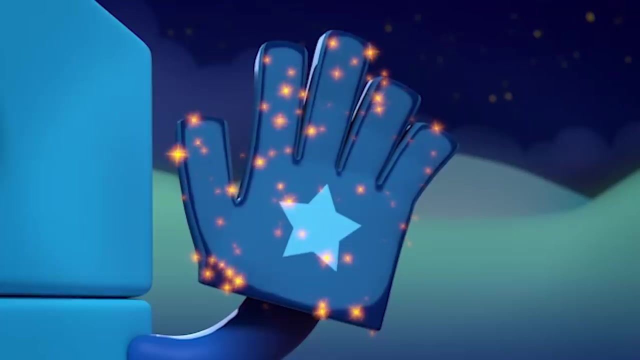 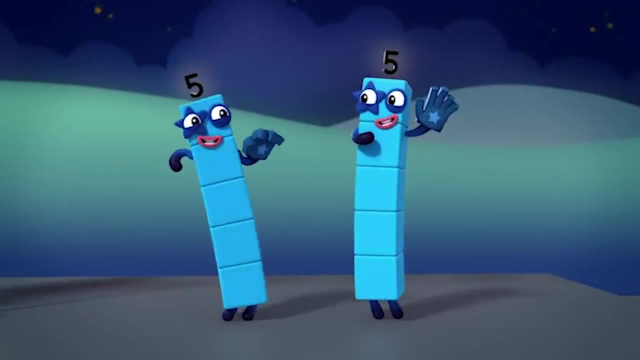 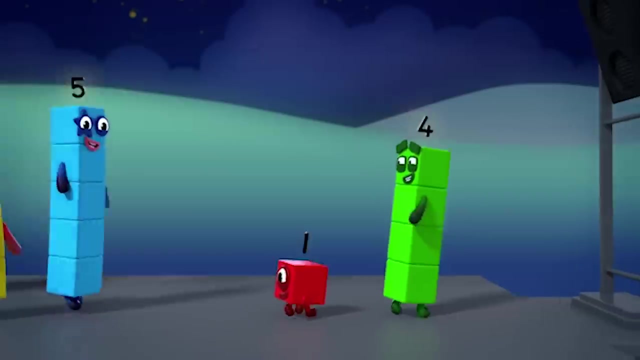 Five points. Oh, a star is born. I don't know about that. Take a look, High five, High five. A big hand for you, High five. Five minus one Equals four. And who are you? I'm five. 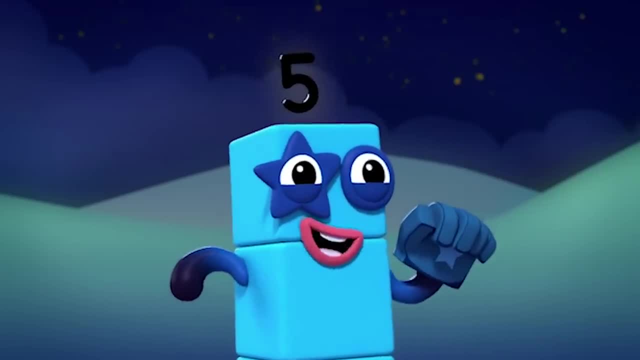 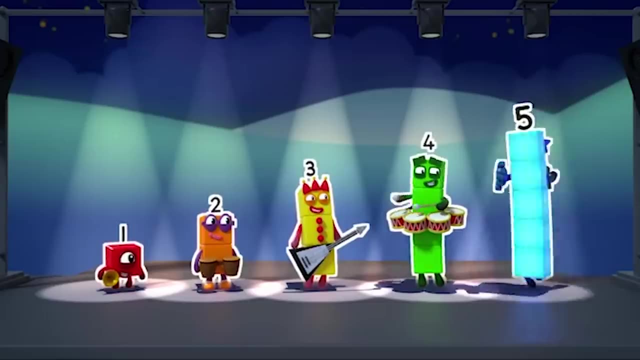 And you can count on me to get this party started. Five members in my band: One, two, three, four, High five, Five fingers on one hand: One, two, three, four, five, High, five, High five. 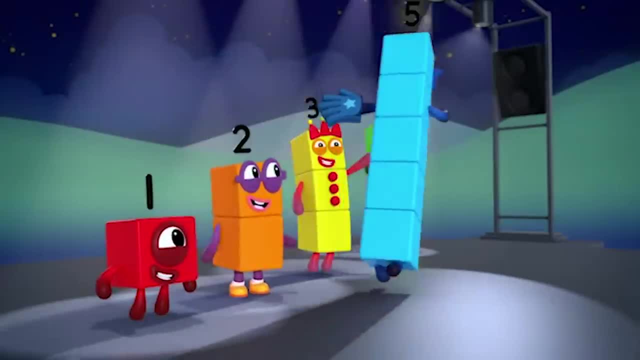 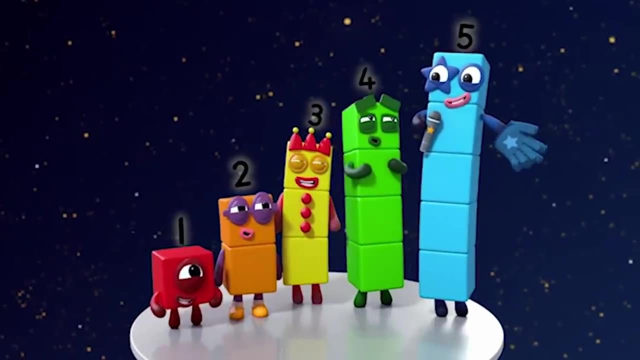 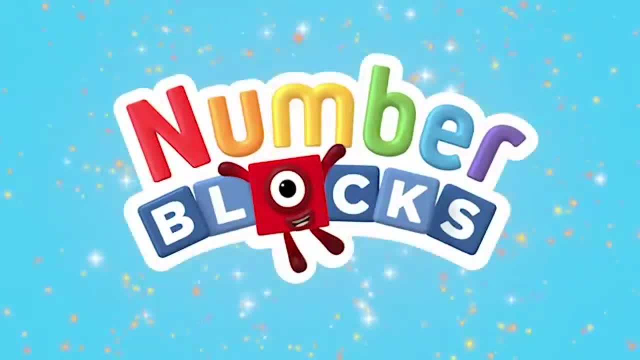 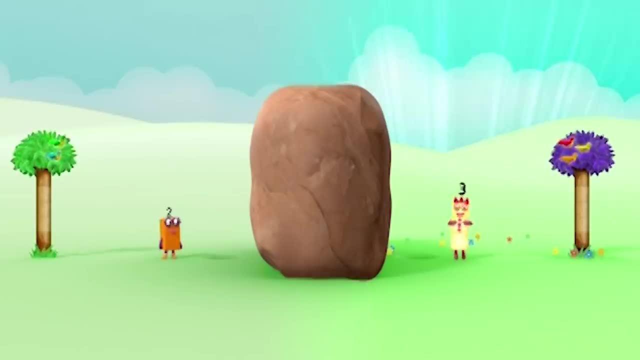 You know that you've arrived. When you're with number five, You can count on us with another box. Now I am two, and here I am. Now I am three and here I am. What a wonderful day to be alive. But where, oh, where, oh, where is five? 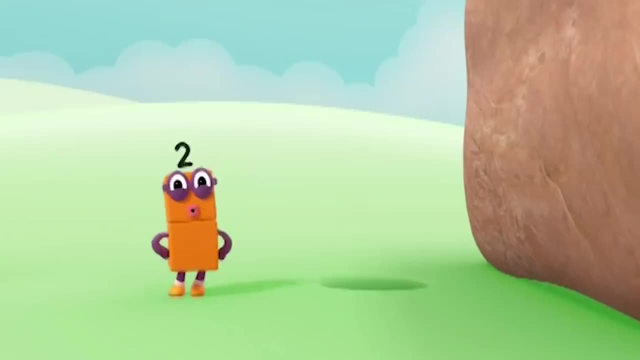 I wonder where the ones will go. I think I've got it Now. I know Every time we get one smaller, someone else is getting taller. What is that silly sucking sound? A giant hole so big and round? Why is it there? 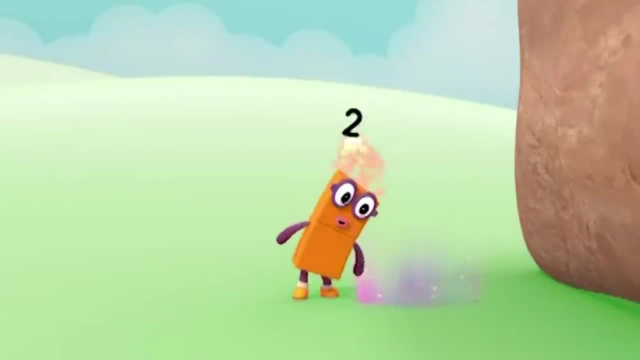 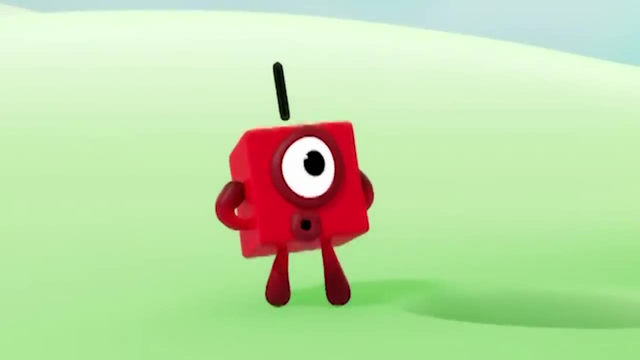 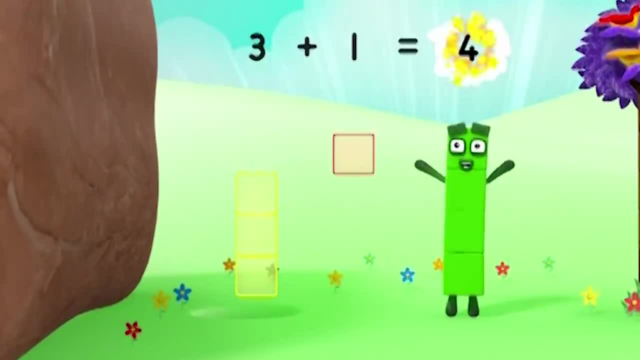 What is happening to me? I just got bigger, Did you see? Now I am one and here I am. Now I am four and here I am. What a wonderful day to be alive. But where, oh, where, oh, where is five? 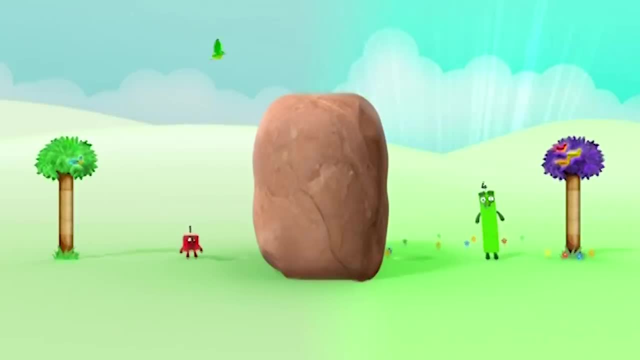 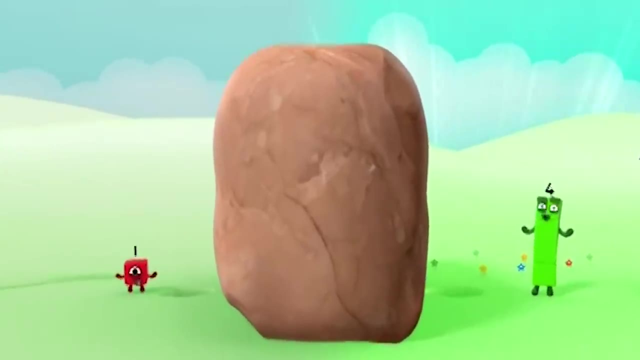 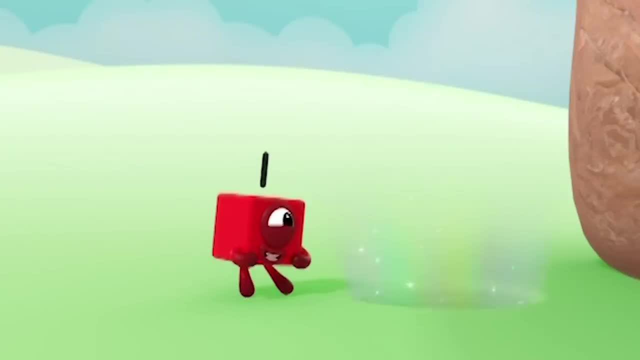 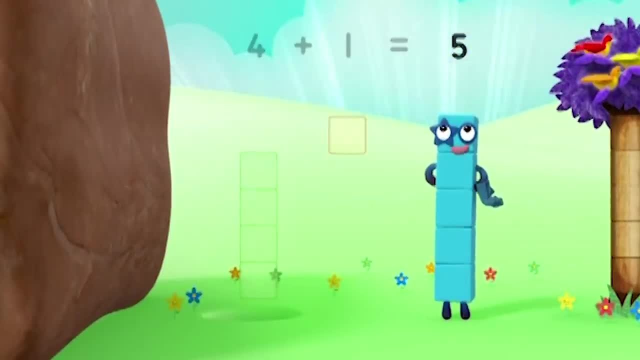 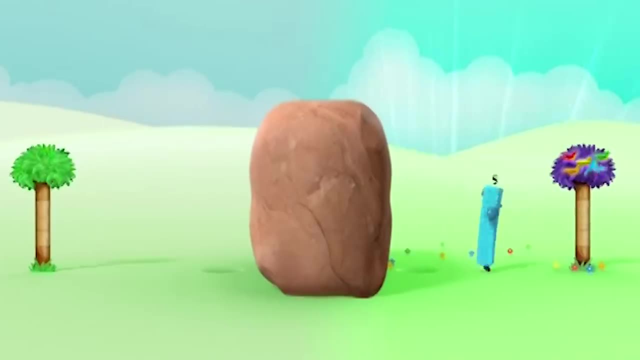 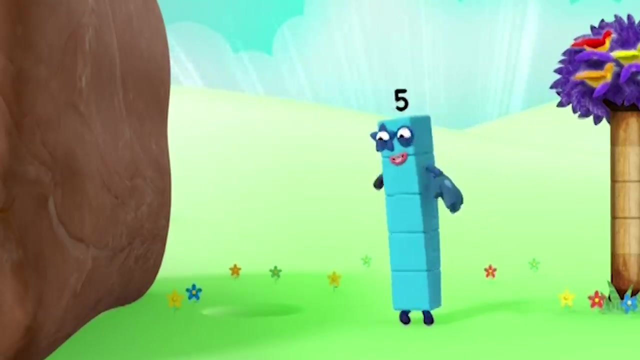 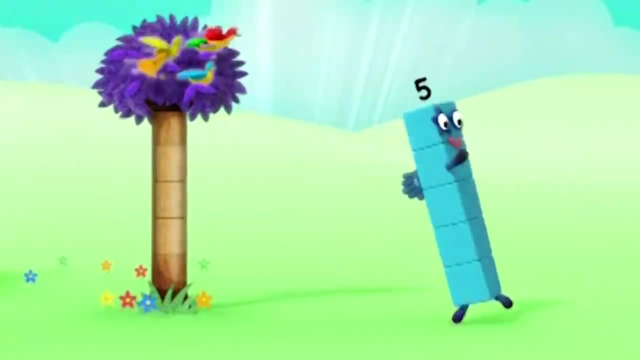 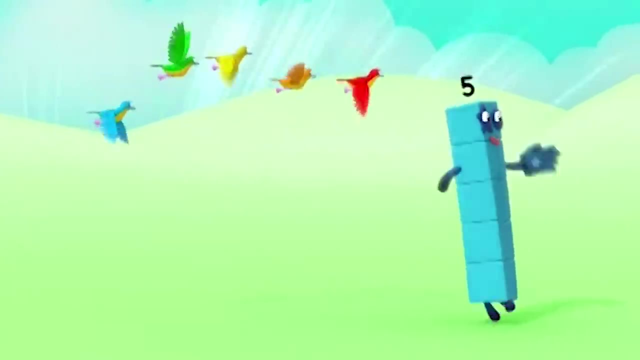 What a wonderful way to arrive. One, two, three, four, five. What a brilliant, amazing, fantastic, terrific and wonderful day to be alive. One, two, three, four, five. You can count on us. we're the number blocks. 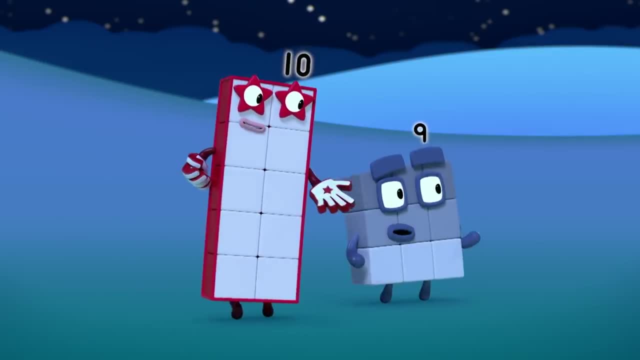 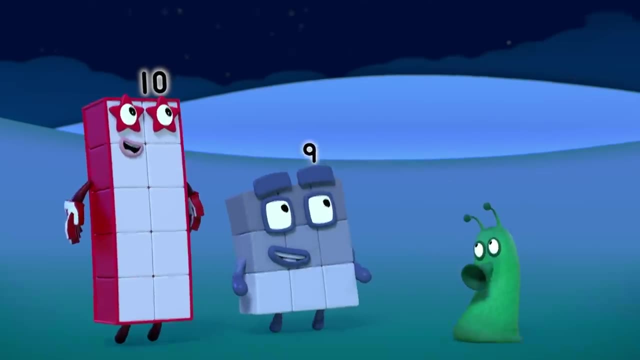 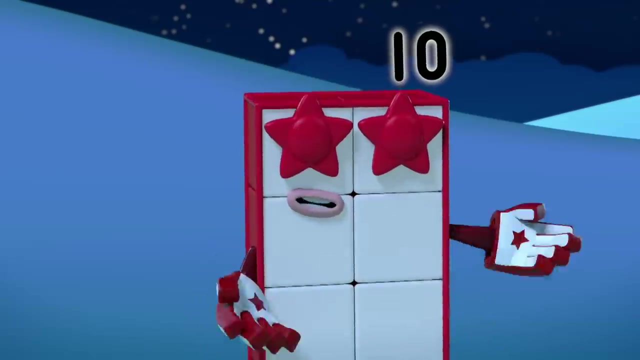 Now there's something you don't see every day: An alien Up up. Ah Look, Is that where you live? Up, up, up up. Don't worry, fellow space cadet, I can rocket you home. 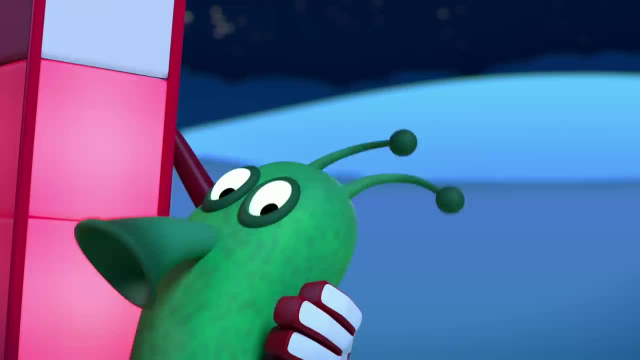 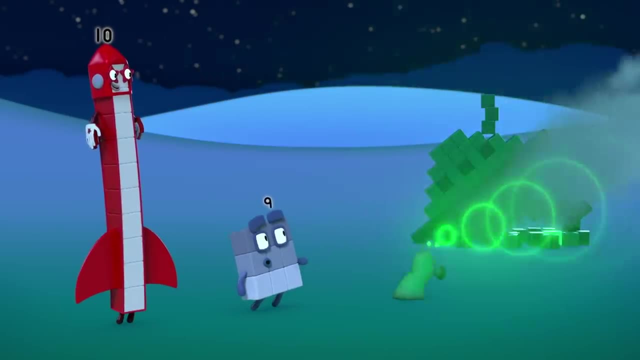 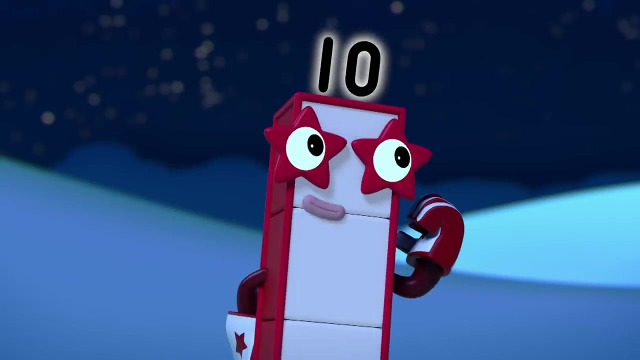 Hold on tight. Ten, nine, eight- Oh, I think she's building a tower Up. Oh, um, I think you'll need more blocks than that. Wolf, Stop That tickles. Oh, Ha, ha ha. 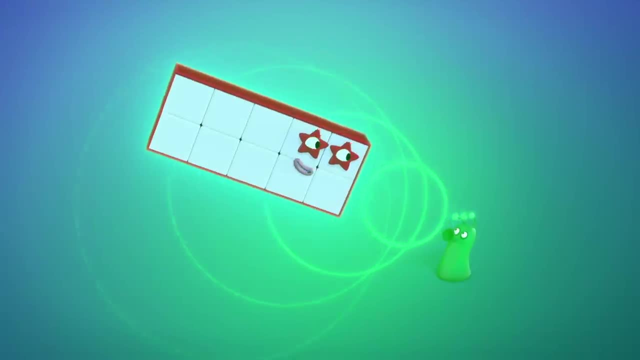 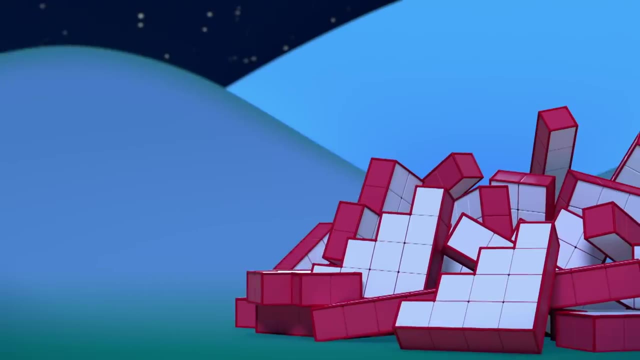 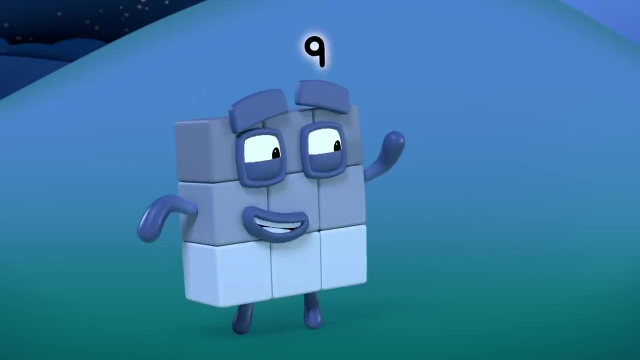 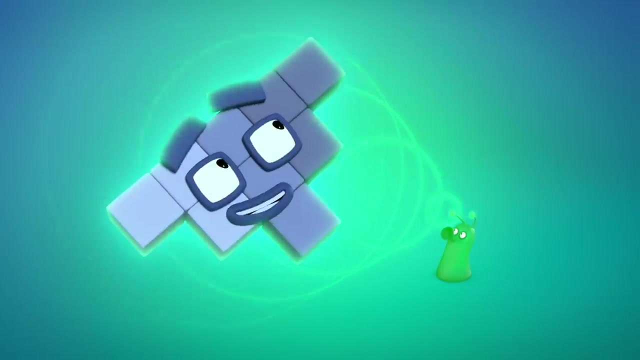 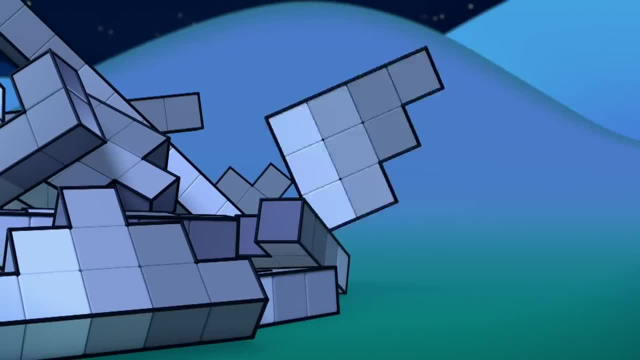 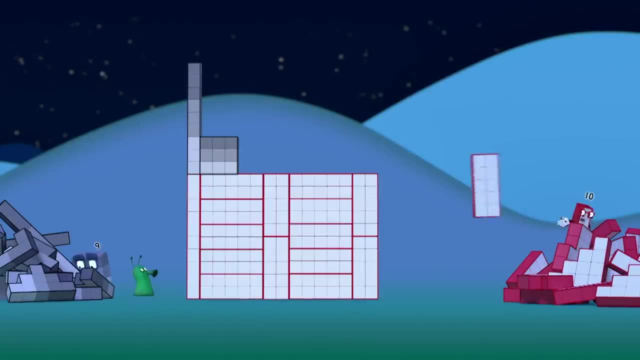 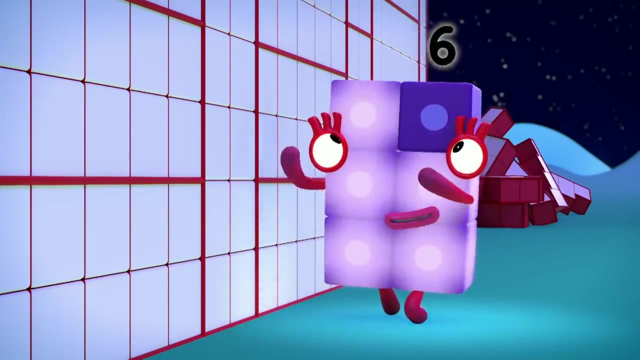 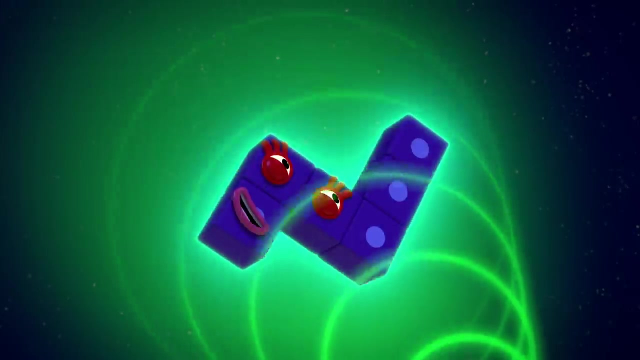 Oh, Oh, Oh, Hey, Can I play One, two, three, four, five, six. Please make me some building bricks. Oh, Ah, Everything looks beautiful. Huh, Oh, slutty me, Ooh. 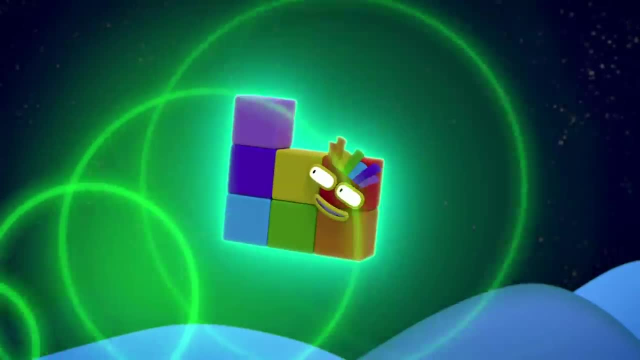 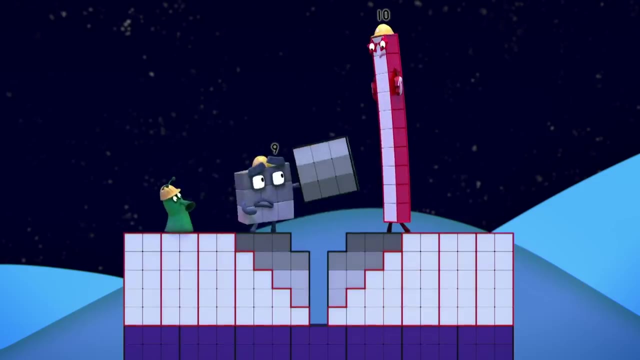 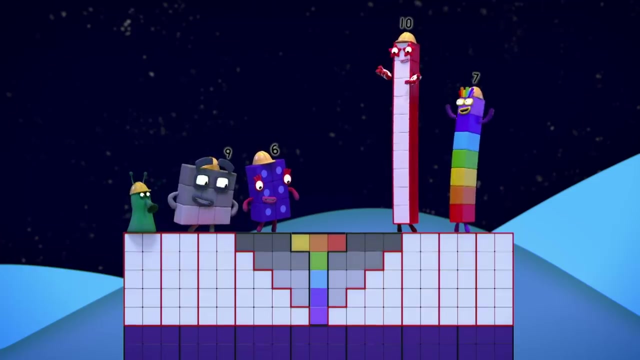 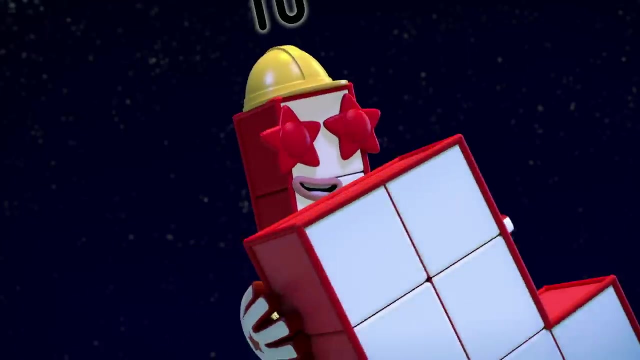 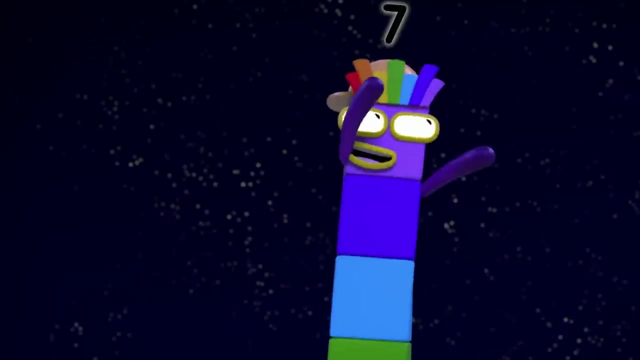 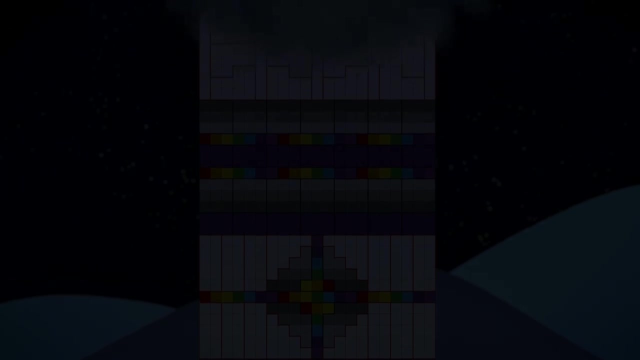 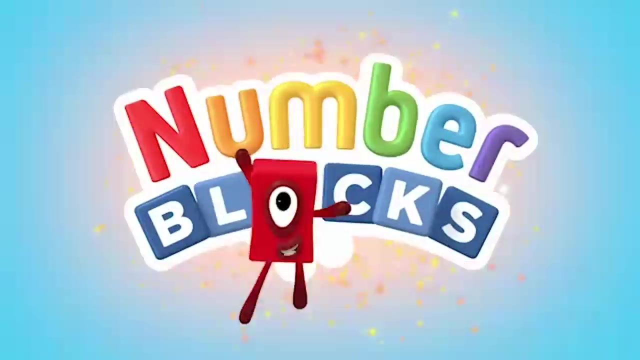 Oh, This doesn't fit, Or this Or that. Try this. Yay, Beginner's luck: Number blocks. let's get building. Oh, Oh, Oh, Oh, Oh, Ooh, Oh, Oh, Oh. You can count on us with another box. 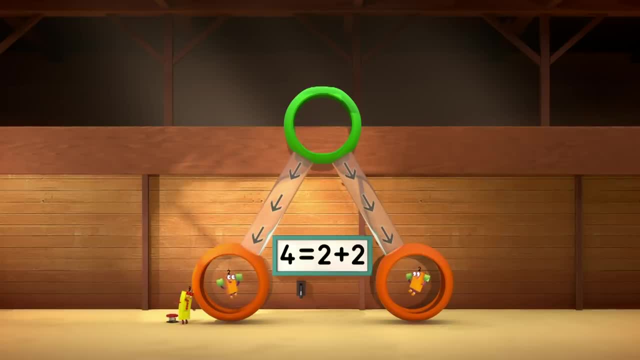 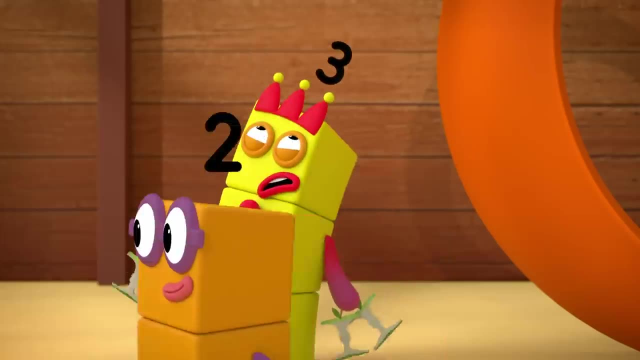 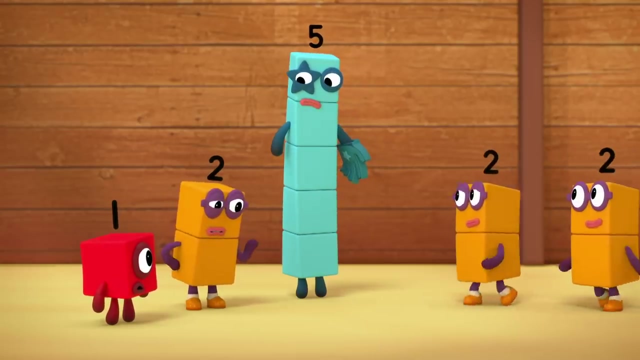 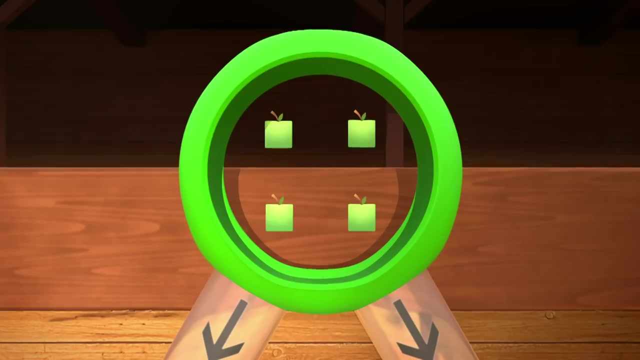 Hmm, Yum-yum, Yum-yum, Yum-yum. No, no, no, You silly machines, Poor three. We need to find a way to make three apples come out. Look, Four new apples at the top. 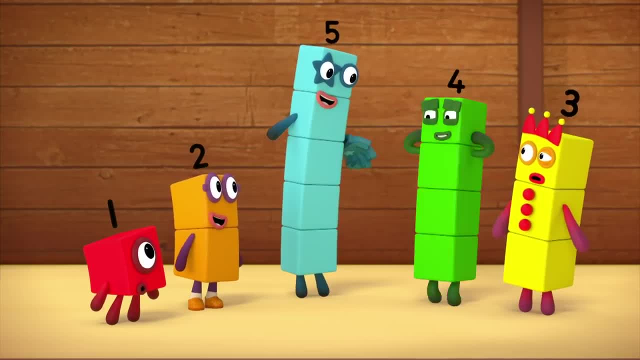 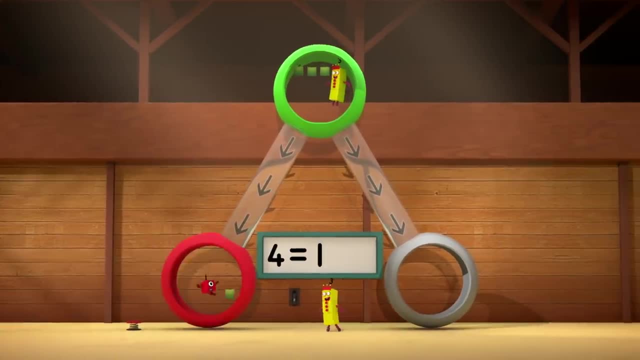 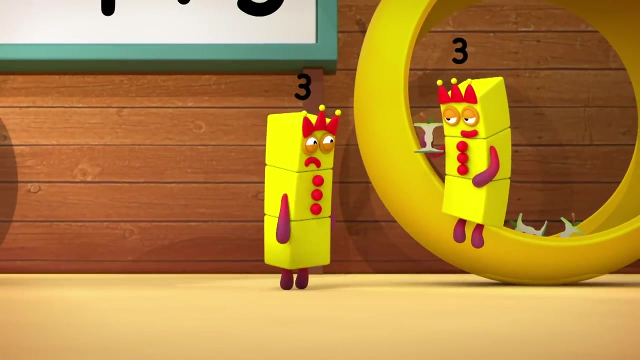 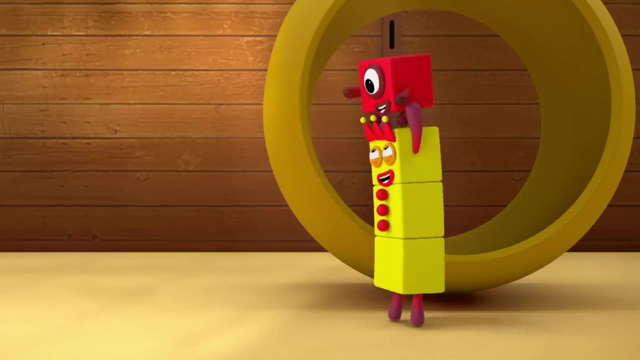 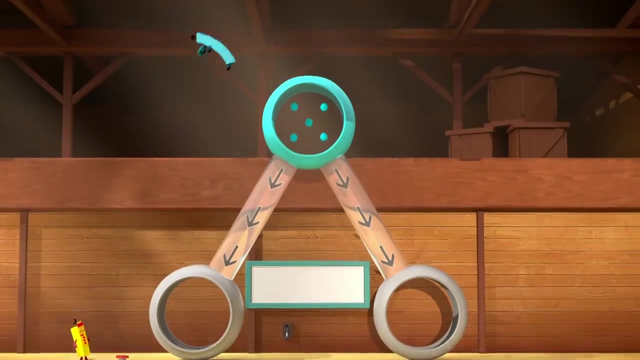 I know how to make three. Here I go. Four equals one plus three. Yes, yes, yes, No, no, no, I won't front. Five equals one plus two. Four equals one plus two. Four plus two equals five.